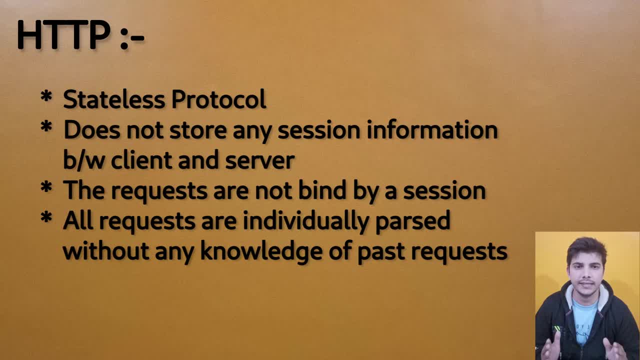 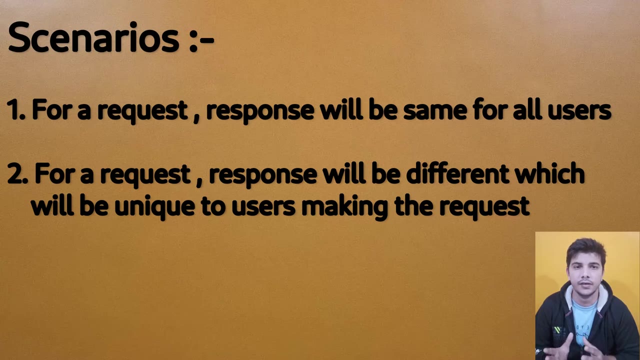 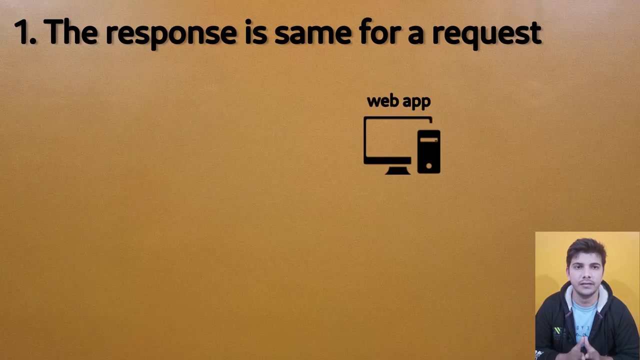 communication between client and server is not bind by a session and no two requests are interconnected in any way. for the server, every requests are parsed individually. now let's take two different scenarios to understand the requirements of cookies for the session management. and the first case scenario. let's say the web application is serving a page which is: 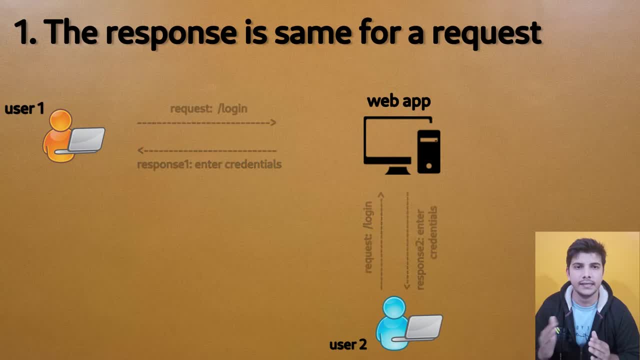 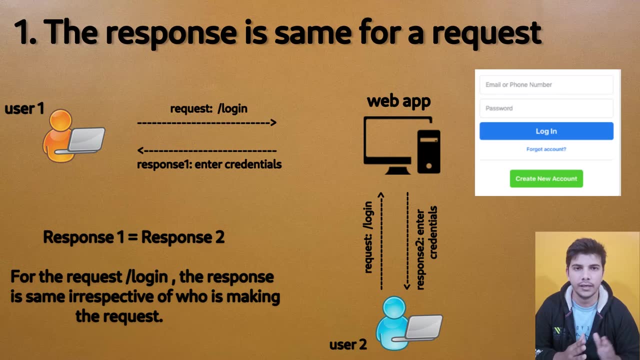 common to all the user or all the client, irrespective of who is making the request, the response will remain the same. for example, consider the login page which is hosted by the website. now for the login page, the response for all the requests will remain the same, even if i make the request, or you make the request, or any other user or any other computer. 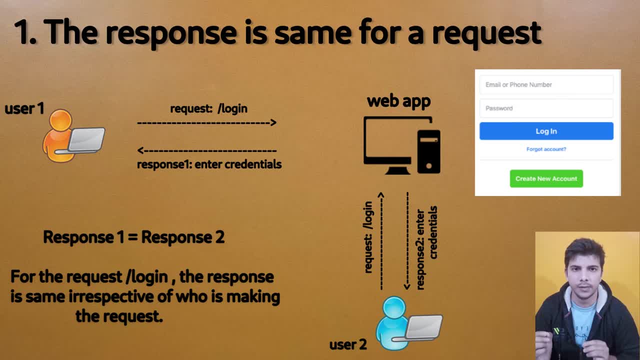 or client make the request, the response will always remain the same. now, in this particular case, the server or the web application is not required to identify each of the requester. so in this particular case, we don't need any session, because for the same request, that is, slash login, the response will remain the same for all the clients or for all the individual user. but 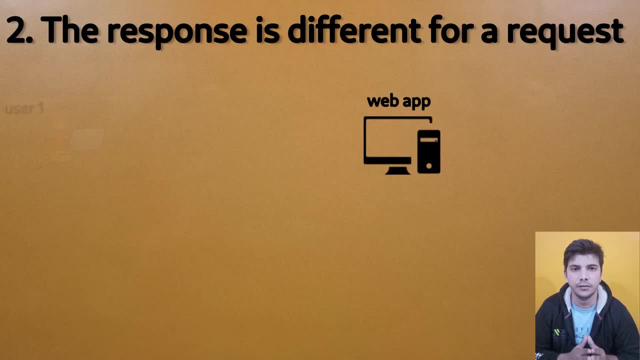 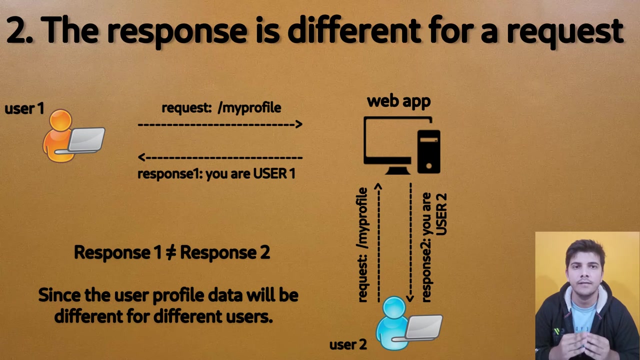 now let's see the another case in which the user needs to get the information about his profile. so he is making the request to slash profile now based on the user or who the user is. the server response, for example, for the request is my profile, then this web application need to return the unique. 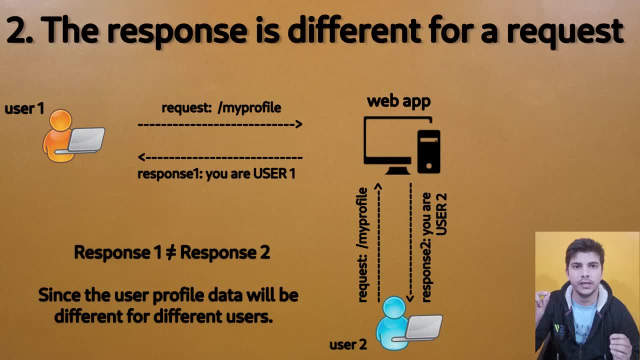 data depending on who is or which particular user is, asking for the data. similarly, if there are three users or four users or any number of users for the same request, that is my profile- the web application is required to send the response based on the user who is asking for the data or asking for the requests. 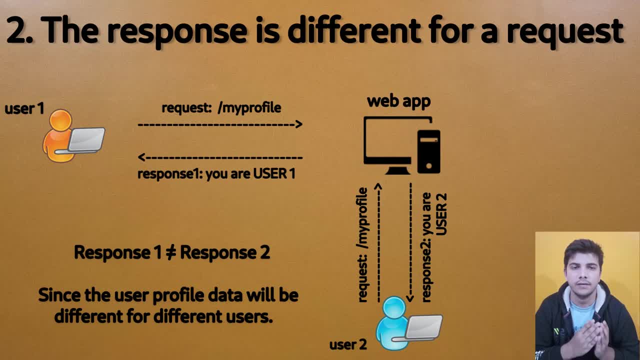 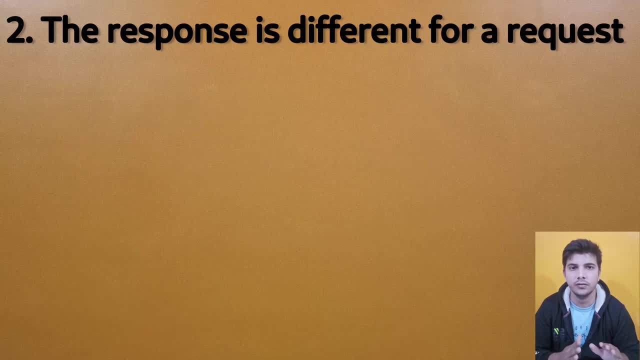 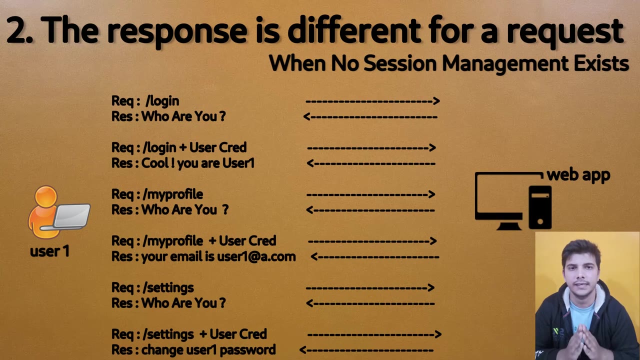 now, in these particular cases, the server or the web application is required to uniquely identify each of the user. now for some time, let's say, there is no concept of session management or cookies. so how it will work. so when i will ask for the page that is my profile, then the server. 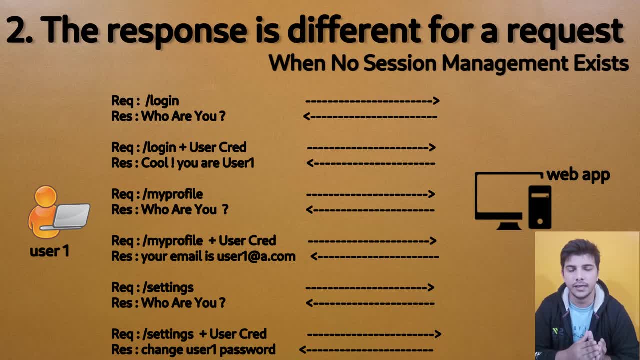 will ask for the username and password once i authenticate to the server. then it will return the response. now, let's say after some time, i need the access to the settings page, so i will ask for the settings, that is, slash settings, and again web application will require. 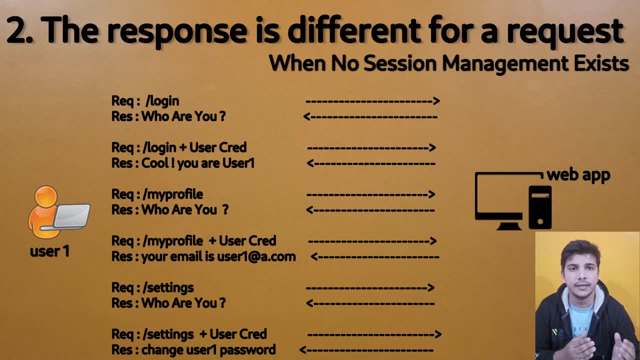 to know who is actually making the requests, since it does not contain any session information. so, again, it will ask for the username and password and then, if we are authenticated successfully, it will give the settings page which will be unique to that particular user. so the point here is that for every request, if the response need to be unique, 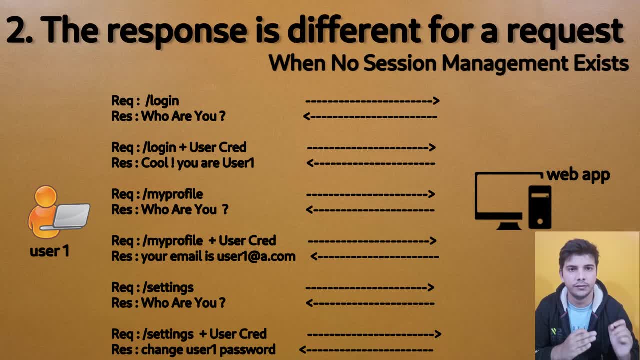 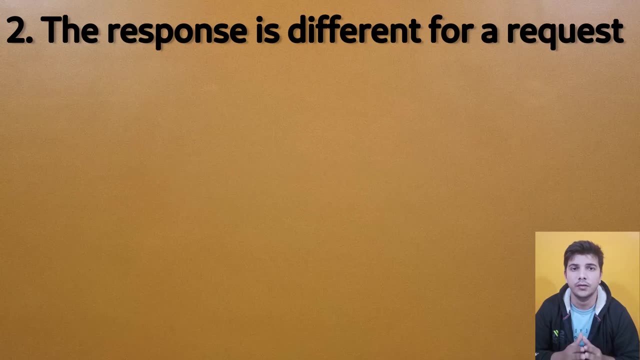 then every time the user will require to authenticate to the web application. so if you request five different things, then you will have to authenticate to the web application five different times. to solve this problem, we have the concepts of cookies in http protocol to understand it. let's start from the beginning. first of all, you will request a page, for example. 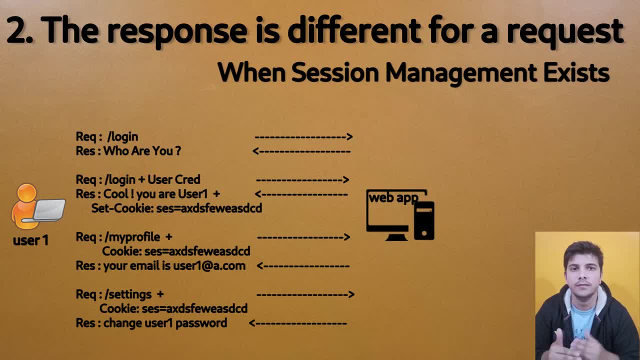 slash login and the web application, in response, will ask you to authenticate to the server or to the web application. now, once you will give the username and password, the web application will check whether the credentials given is correct or not. if the credentials are correct, then it will generate a random string which is known as the cookies in our case. 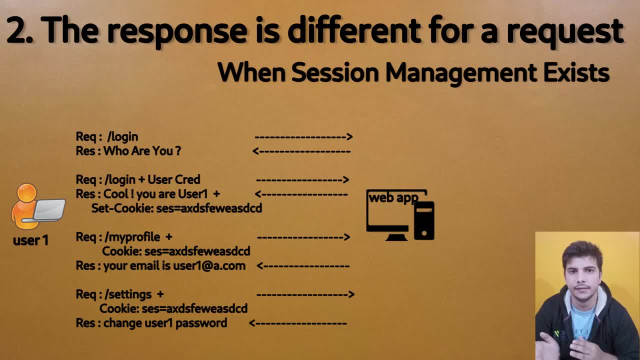 and it will send the cookies in the response headers. now, along with creating the cookies, it will create an entry in a database stating that this user has this particular cookies. so whenever, in any request in its header, if this cookie is coming up, it means this particular user- that is, the cookie associated with that user- is asking for the data. now another point. 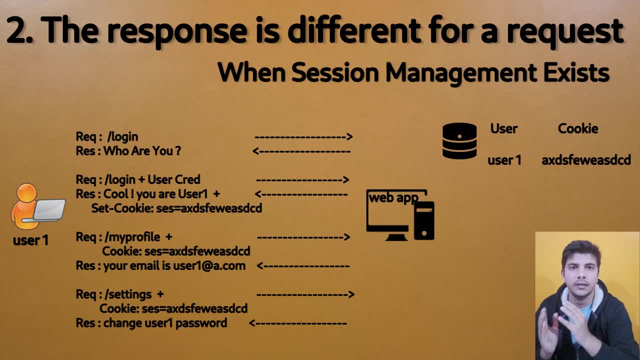 when the web application send the cookies to the browser, then the browser store it into its memory. all right. so next time, let's say, we are making the request to the my profile. so in that case, what browser will automatically do? it will get that cookie and send it to the web application.